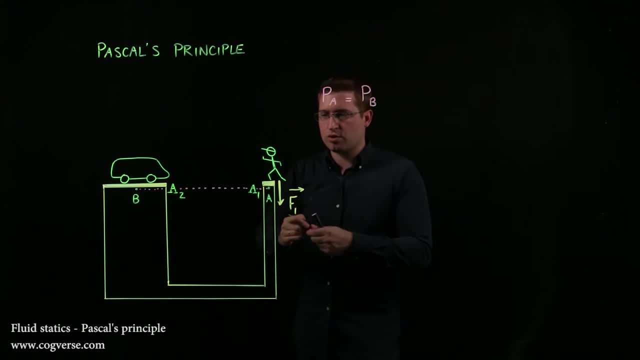 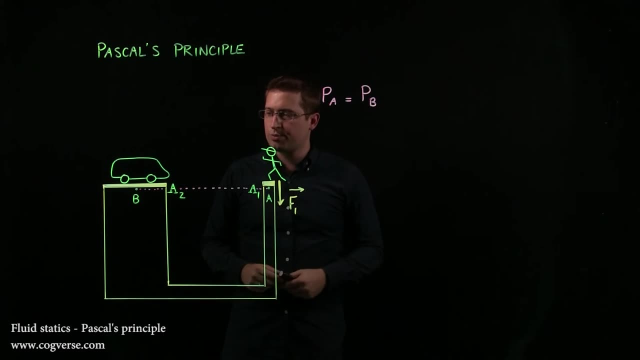 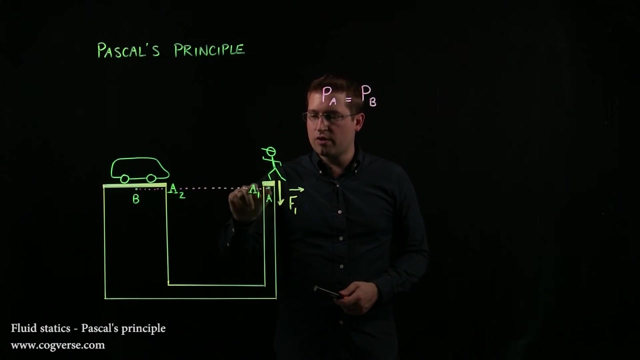 is equal to the pressure at point B, because there are two points in the same fluid at the same height and the fluid is at rest. Therefore PA equals PV. But that's not bad right, Because when the mechanic exerts a force F1 over the area A1,. 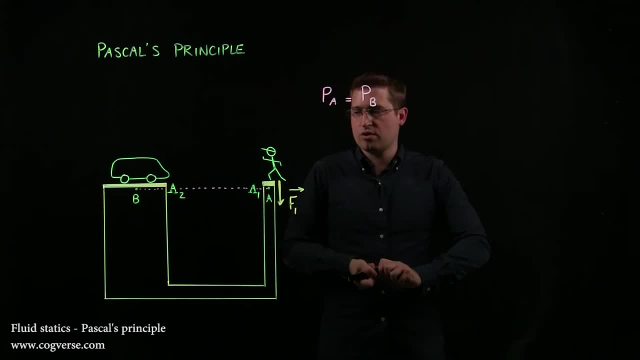 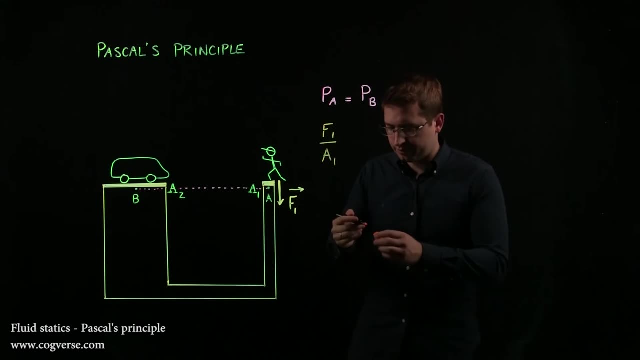 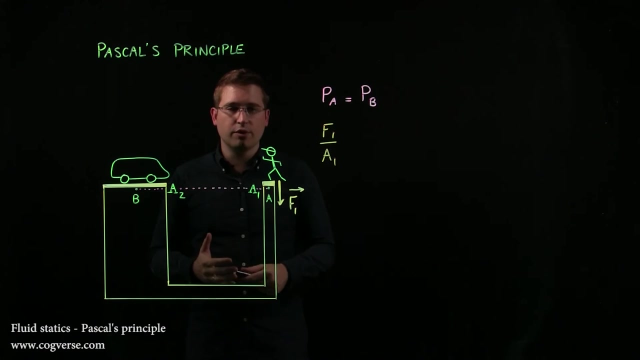 then the pressure here, or the increase in pressure we should say, is in fact F1 over A1., And that increase in pressure is immediately transmitted to every point of the fluid without any loss. In other words, PA will be equal to PV, or the increase here will be the. 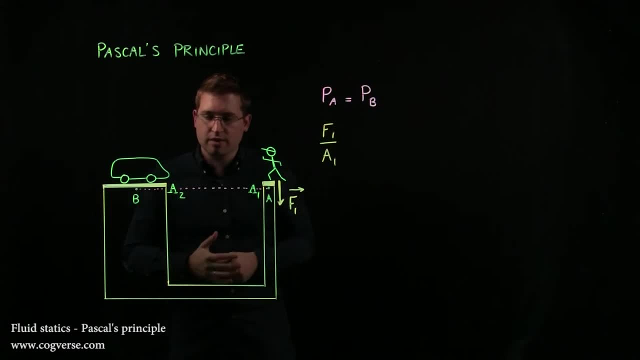 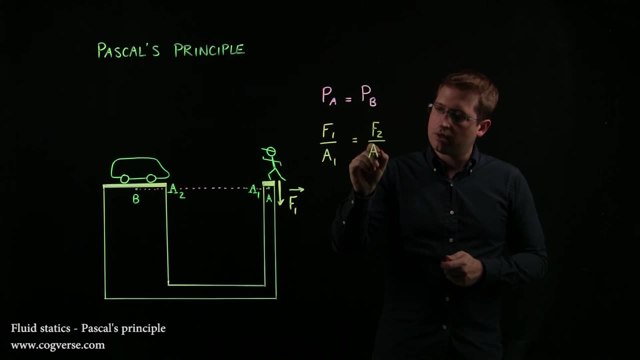 same as the increase here, And here our pressure is going to be F2 over A2, because the force F2, which is directed upward, is going to be F2 over A2, because the force F2, which is directed upward. 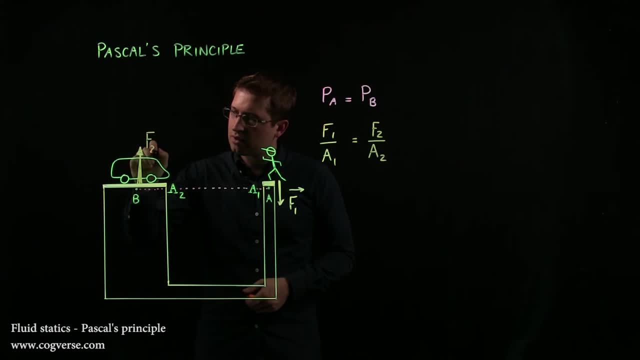 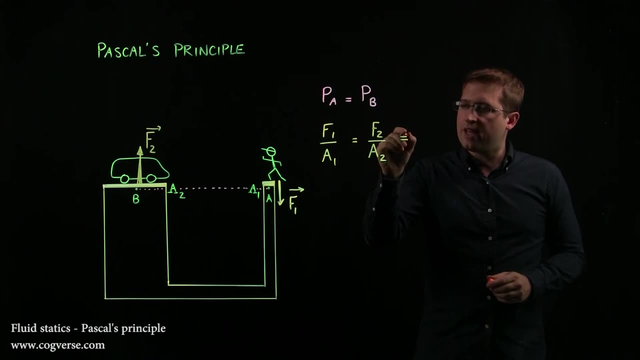 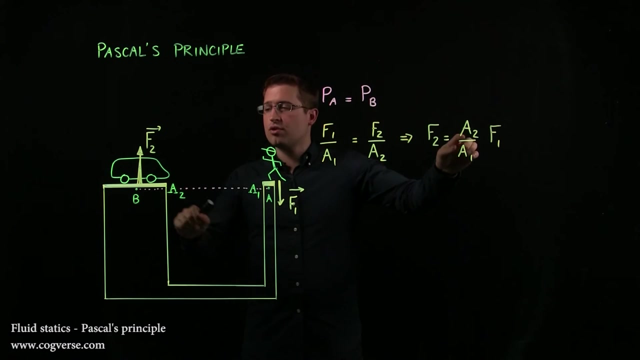 is the force that comes from the fluid pushing on this area A2.. Now that means that F2 is equal to A2 over A1 times F1. And what it really means is that if I make A2 really big compared to A1, this ratio here: 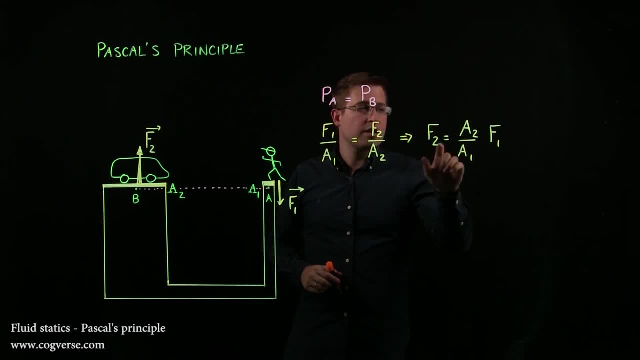 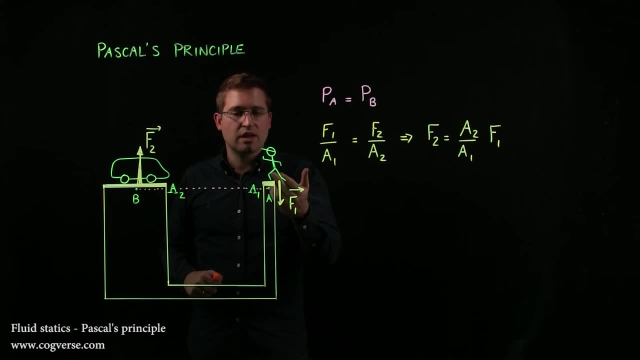 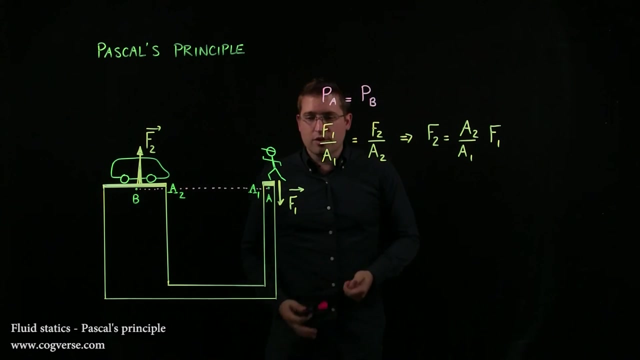 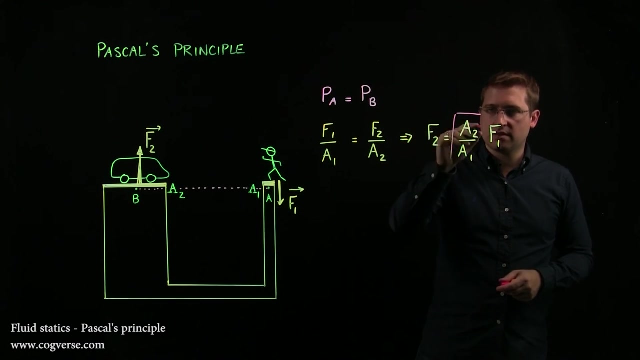 is going to be huge, And therefore F2 can be much bigger than F1.. And by here exerting a force that's a reasonable force for a mechanic, I can in fact lift a car, which is pretty impressive. So that is an example of Pascal's principle. And just for the sake of naming things, this ratio. 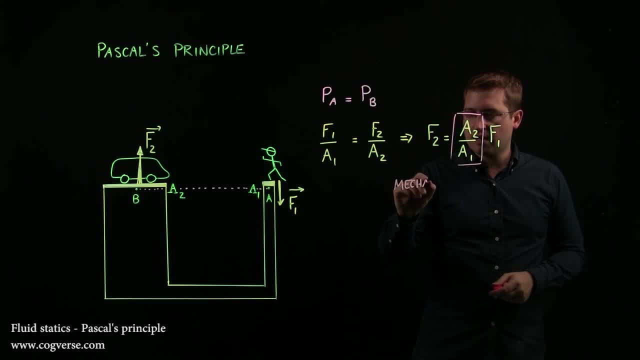 here is called the mechanical ratio, And I'm going to show you how to use this ratio. So I'm going to show you how to use this ratio And I'm going to show you how to use this ratio. 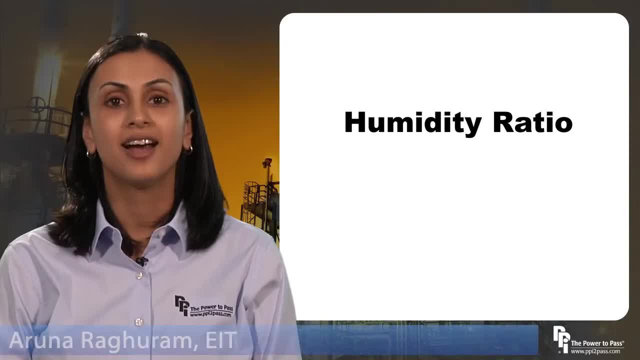 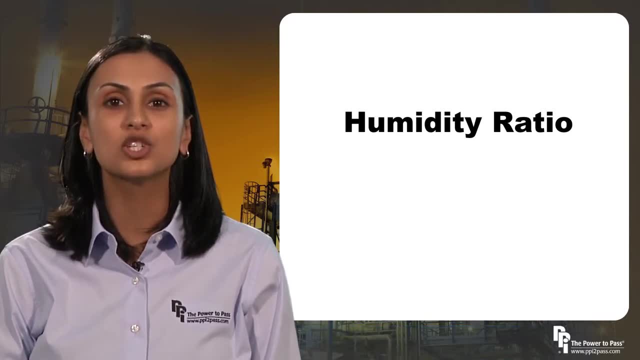 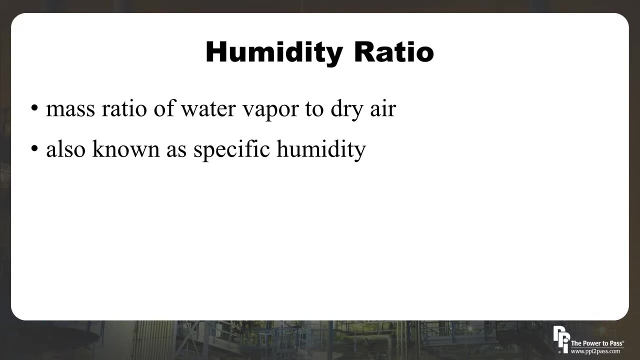 Hi, in this module let's talk a little bit about humidity ratio. The humidity ratio is defined as a mass ratio of water vapor to dry air, and this is also known as specific humidity. Now humidity ratio is used to specify the amount of water vapor contained in atmospheric air.